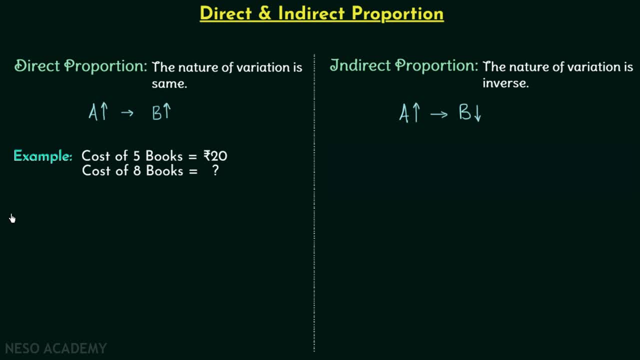 to find the cost of eight books. Let us say that the books is our quantity A and the price for the books is our quantity B. Now what type of proportion we have in this case? Initially we have quantity A as five. then we have quantity A increased to eight. Quantity A is equal to: 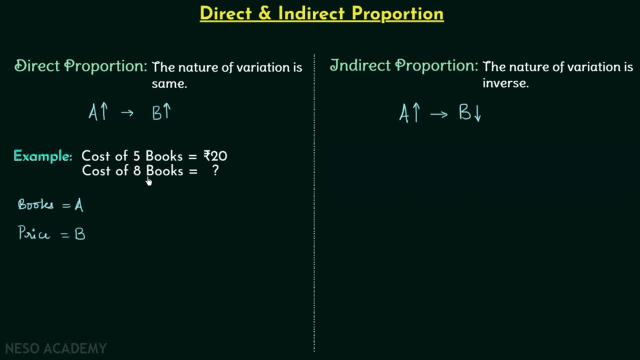 quantity B. Quantity B is twenty and when you increase quantity A, that means when you increase the number of books, what will happen to the price, the quantity B, The price will also increase. It is obvious. The price will increase. It will be more for eight books than five books. So when you are 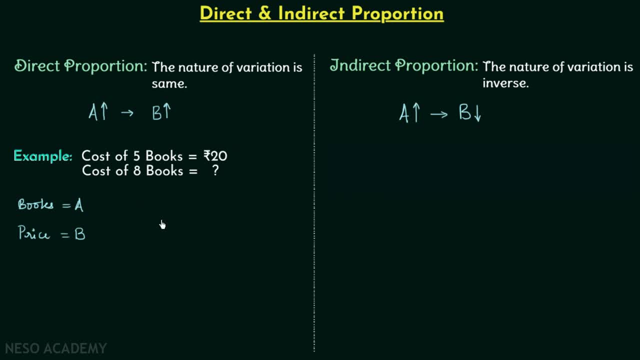 increasing A, B is also increasing and therefore we have direct proportion between books and price. So we will have A proportional to B, and we know this sign. This is the sign of proportion. Now we also know that when we remove the sign of proportion, we multiply this quantity by constant. So if I remove it, we will have equal. 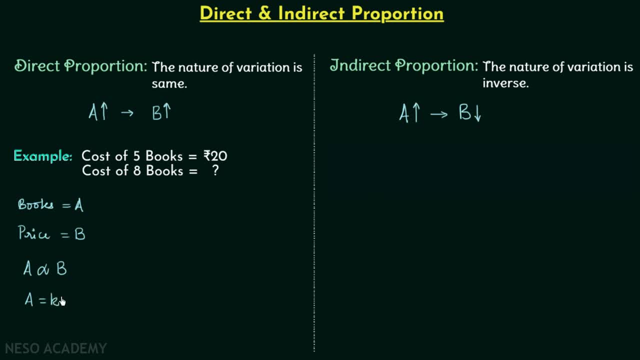 to in place of it and we will multiply constant. let's say K to B. From here we will have K. K will be equal to A divided by B. Now this constant K will remain same for different values of book and prices. So I can say, if we have A1 over B1, we will have same constant, or if we have A2 over B2,. 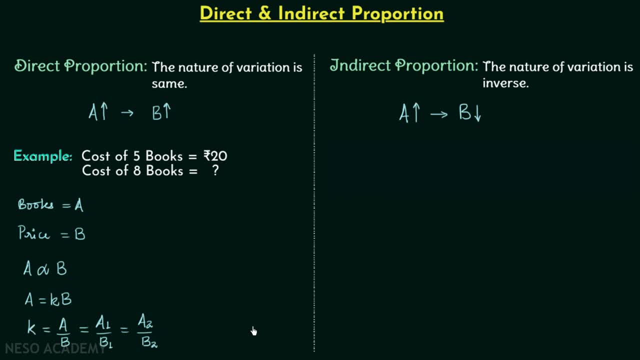 we will have same constant and so on. Now focus on these two: A1 over B1, equal to A2 over B2.. From here we can have our price: A1 is equal to 5, B1 is equal to 20, A2 is equal to 8. 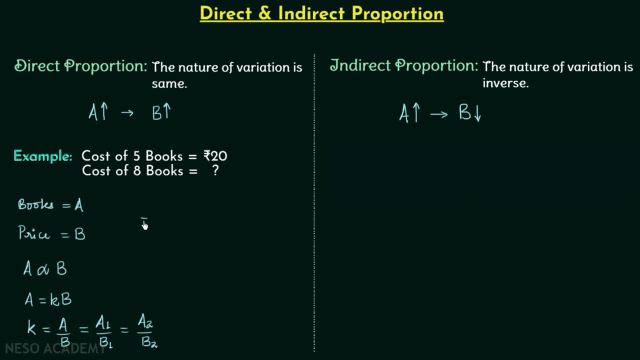 and B2. we need to find out. So we will have 5 divided by 20 equal to 8 divided by x. Let's say the price we need to find is equal to x. From here we will have x. x will be equal to 20 divided by 5.. 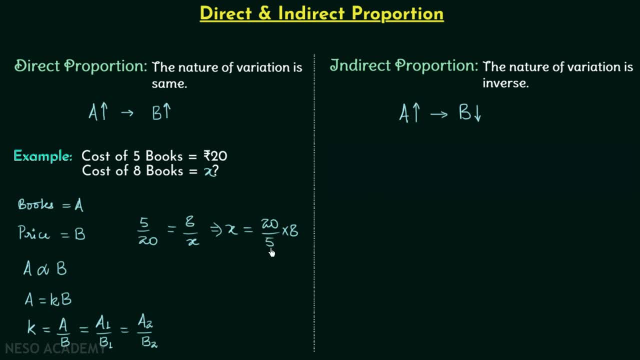 Okay, Okay. So 20 divided by 5 is equal to 4,. 4 multiplied to 8 will give you answer as 32 rupees. So 8 books will cost you 32 rupees. So I hope you now understand the example of direct proportion. 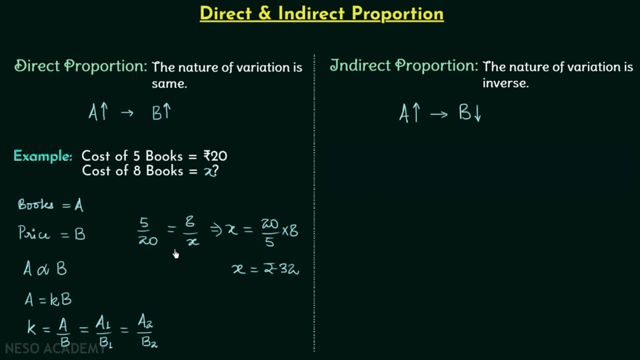 The same answer you can have following the unitary method as well. 5 books is equal to 20 rupees, So 1 book will be 20 over 8.. 20 over 5 rupees, and therefore 8 books will be equal to 20 over 5 rupees multiplied to. 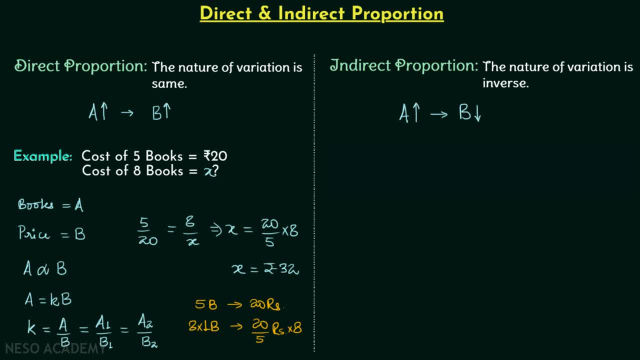 8, giving us 32 rupees. So in this way we are done with the direct proportion. and now we will move on to the example problem of indirect proportion. In this problem we have a piece of work and 5 men are doing this piece of work in 10 days. 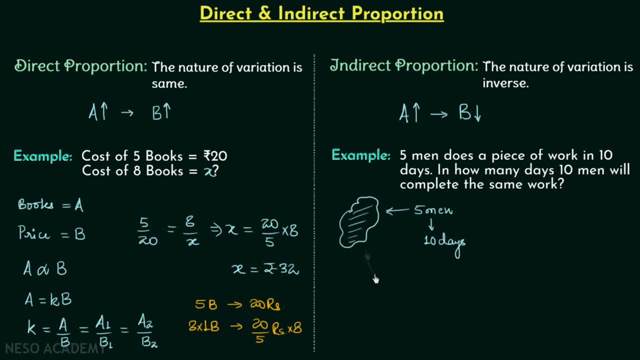 We have increased the number of men. We now have 10 men. We now have 10 men to complete the same piece of work, and this time we need to find how many days 10 men will take. So what do you think? The same work is being done by 5 men and 10 men. 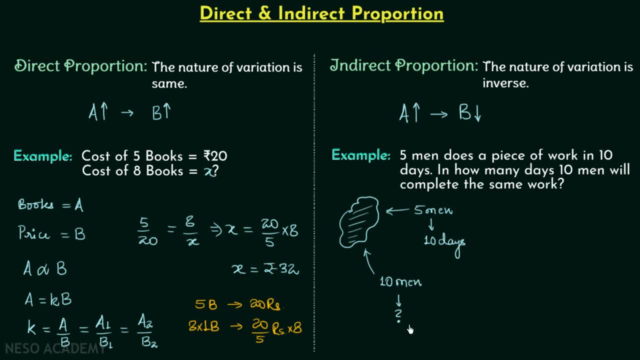 5 men are taking 10 days, and 10 men will take how many days? It is certain that 10 men will take less amount of work. So quantity A is increasing. Initially it is 5 and then it is 10.. Quantity B will be decreasing. 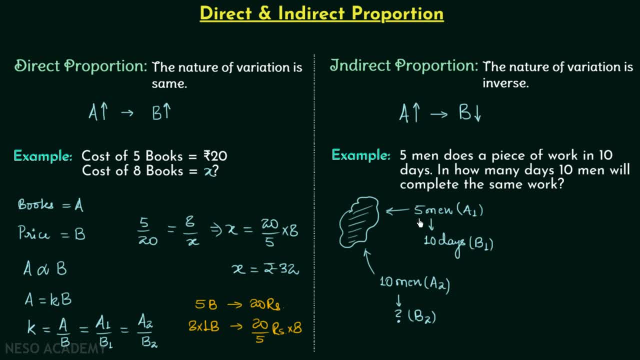 Initially it is 10 and later it will be less than 10.. So A is increasing, B is decreasing and therefore we have indirect proportion in this case. Now let us shift our focus on finding out The number of days 10 men will take to complete this work. 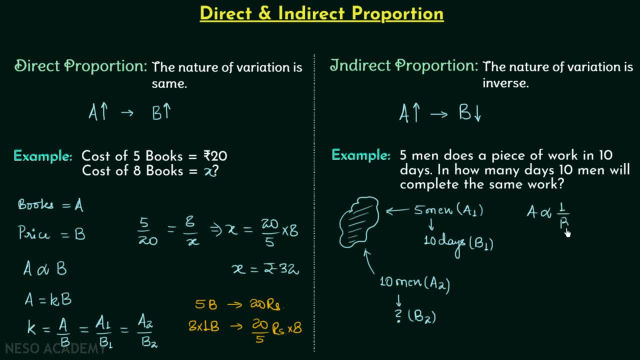 We know they are inversely proportional. So we will have proportionality sign and the other quantity will be inverse. Here it was not inverse because we had direct proportion and here it is inverse because we have indirect proportion. Now again, we will remove the proportionality sign.